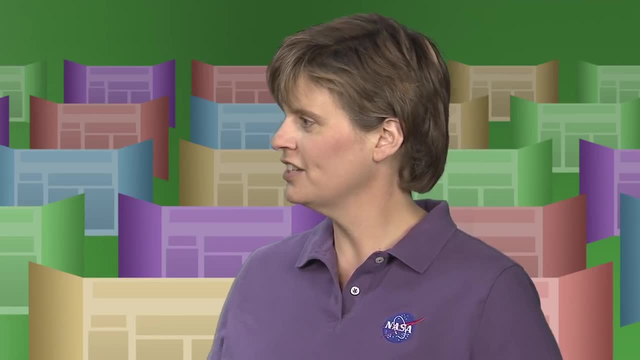 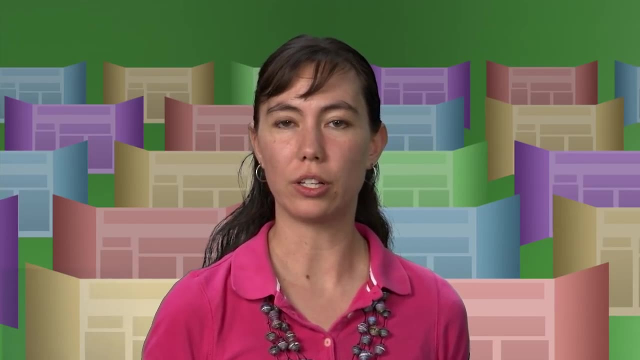 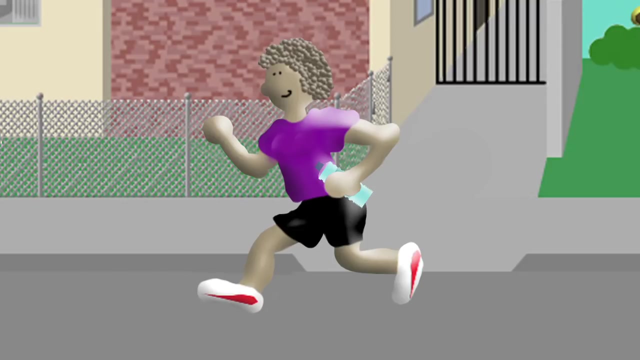 take another example from the original drawing that she identified as something she could ask a question about. So I brought up the example of an experiment looking at how you can improve someone's jogging, For instance. let's consider the science question of how the amount of water that you drink. 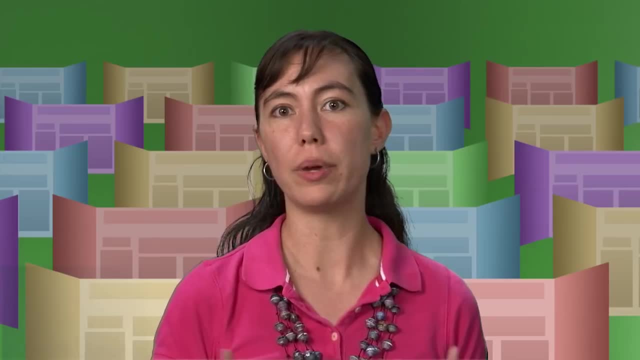 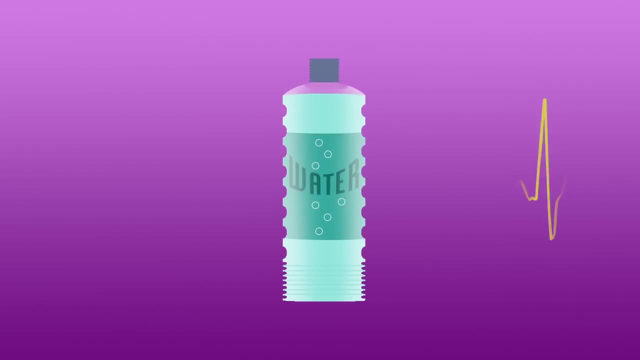 before a run impacts how hard you have to run, And the measurable we're going to use for the output is your pulse rate, and then the input variable would be the amount of water that you drink. Again, we just want to be testing one variable: the effect of 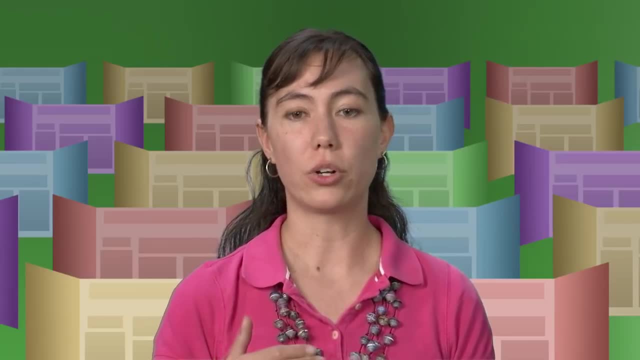 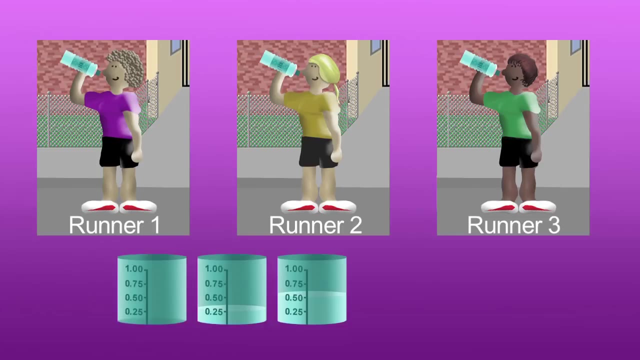 one variable on someone. So you want to make sure that you have people drinking water the same amount of time before the run and the only thing that you're varying is the amount of water. So let's assume that you collected all of that information and you've put it up on. 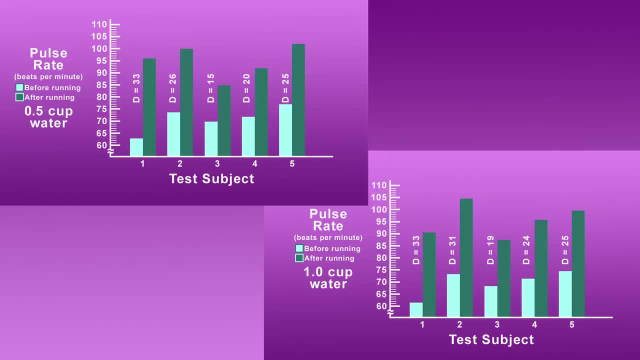 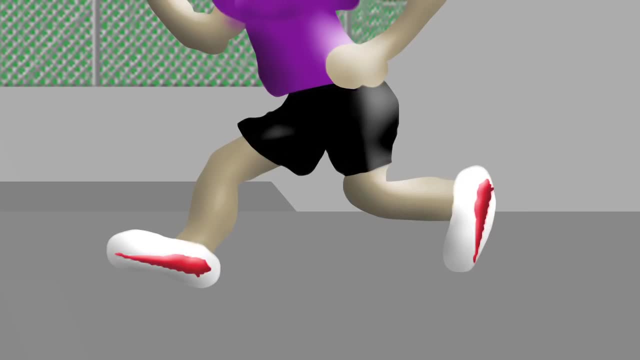 a plot. You've had several different people drink, for instance, maybe half a cup of water 10 minutes before running, or one cup of water 10 minutes before running, And then you had them run a certain distance and then you took their pulse rate. at the end There might 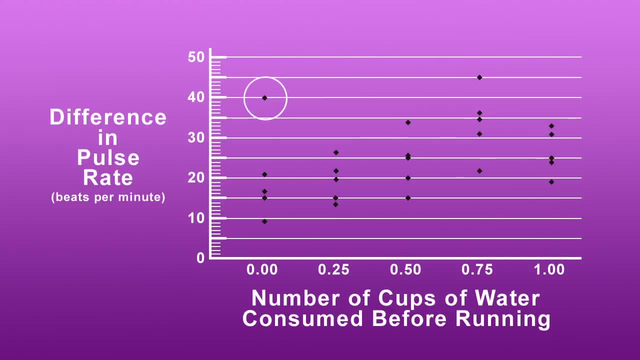 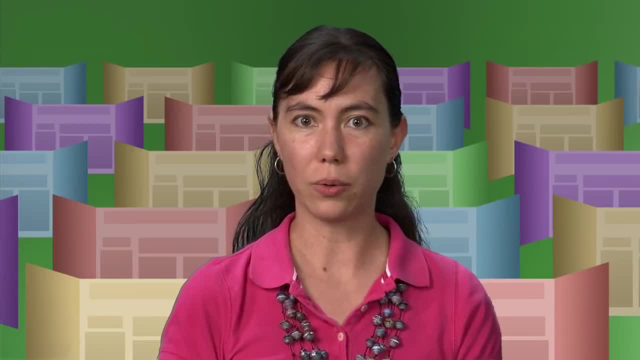 be one person that when you look at the results, they're going to have the same amount of water as you. So these results don't quite fit the trend. You expect a certain trend and as you look across these people, there's just one person that stands out. So then you have to ask the. 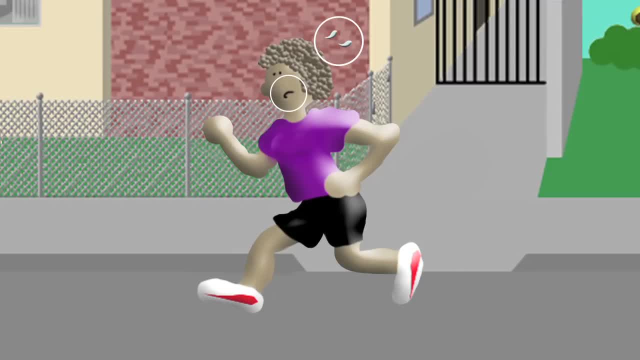 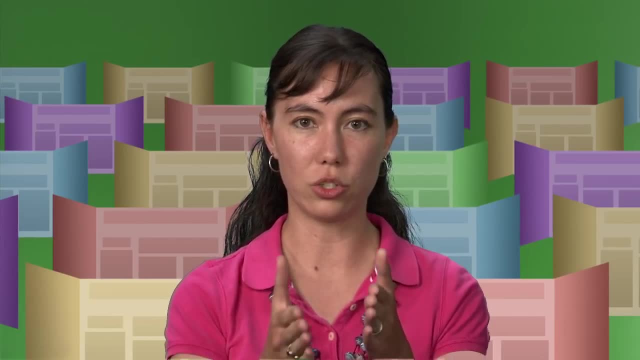 question: were they particularly tired during one of the runs? When you took those measurements, was it at a different temperature? perhaps As much as we try to keep the experiment just to one variable, other things can come in and complicate the results. 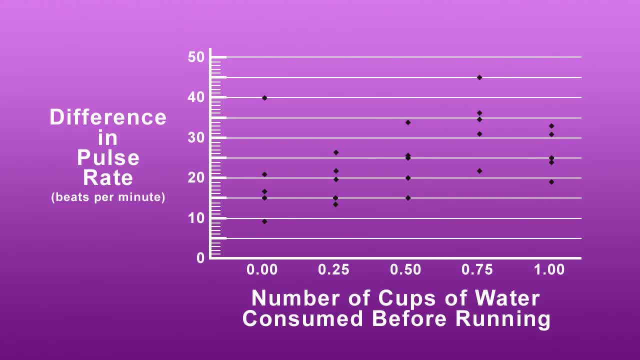 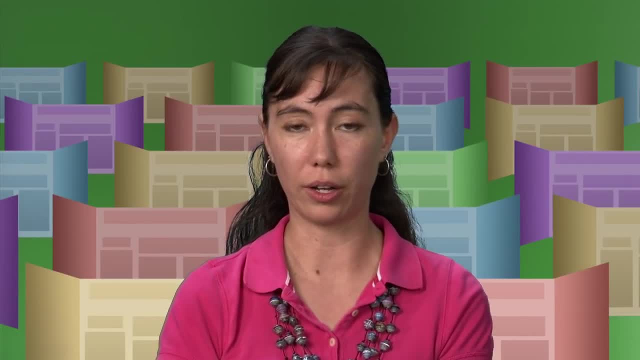 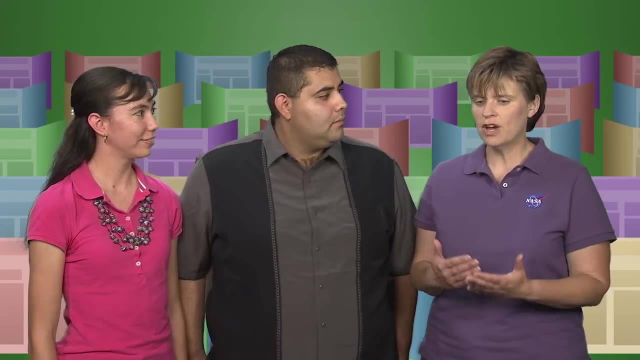 So hopefully you've collected enough data that overall you see something that explains and either confirms or shows that your hypothesis was wrong. But that anomalous data you need to make sure that you can explain it All right, And so it doesn't really matter if your hypothesis is proven or disproven. 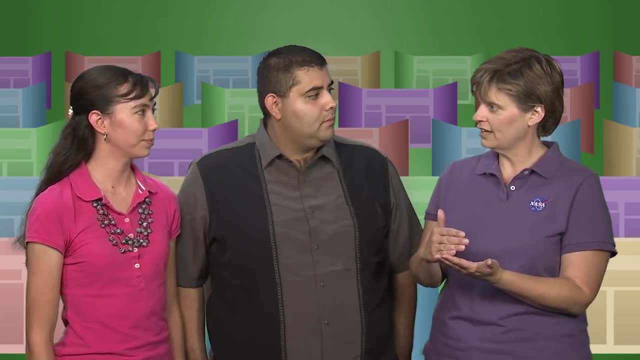 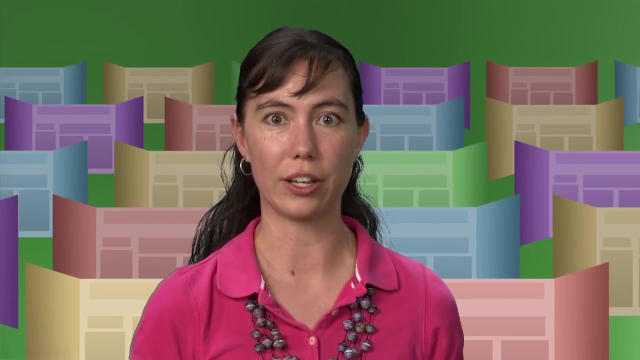 It's a matter of whether you have looked at all the facts, all the data and examined some of the external factors to explain your data. Mm-hmm. Yeah, you definitely want to have collected enough data to actually try to answer whether or not your hypothesis was correct or wrong. 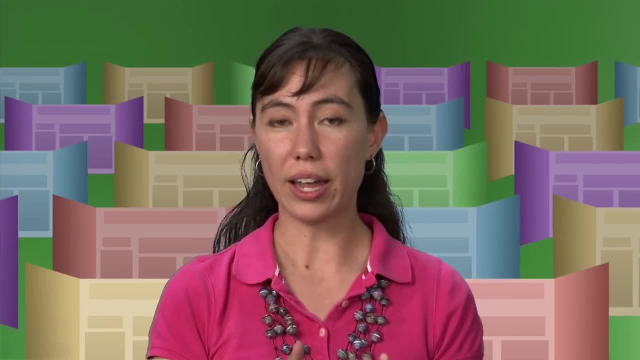 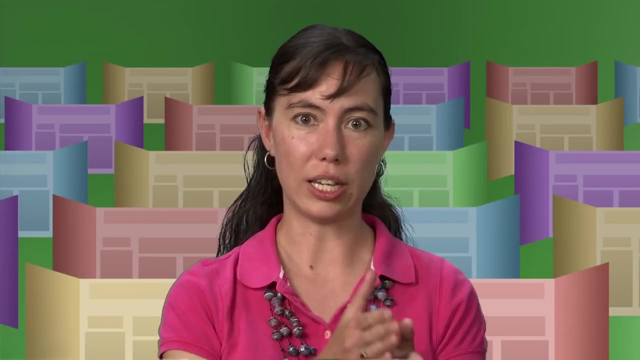 But even saying no, my hypothesis was wrong. that is a result, And that's a perfectly acceptable result, as long as that's what your data shows. And then, just if there's any extra little bits, a data point that doesn't quite fit when you'd graph it up, you just need to have 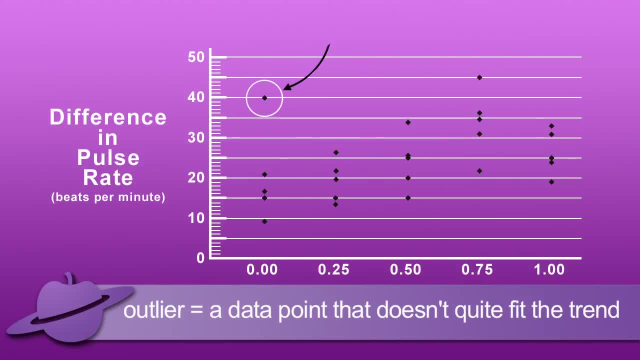 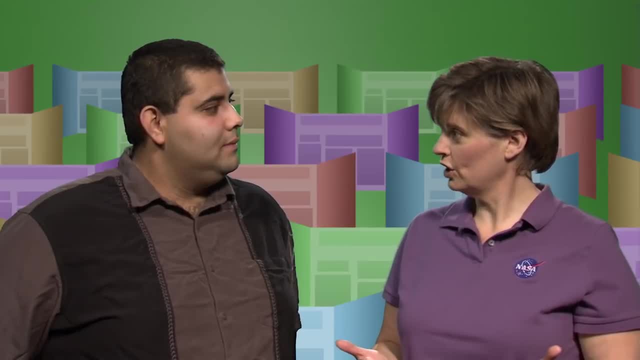 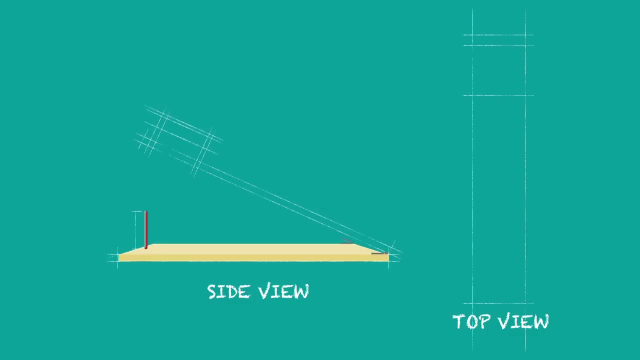 an explanation for why that point doesn't quite fit in with everything else. So, Arby, you mentioned this free throw machine. I don't have any idea how that would look. Can you explain that to me? Definitely, Um. The way I would build it is: first get some plans, draw it out. You'd have a wood frame. 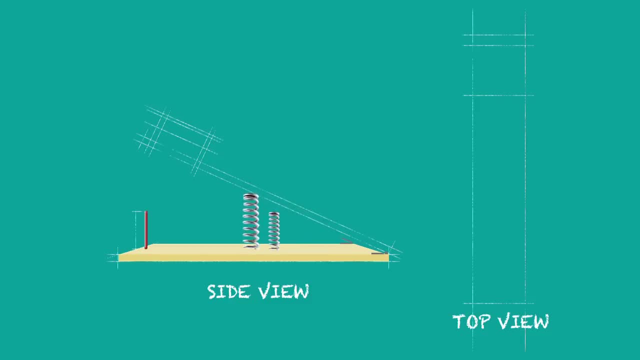 You'd have a couple of springs to provide the energy needed to launch the basketball. You'd need a lever arm to cause the action of shooting a basketball. It's a pretty basic build, so it's mostly important to get it down on paper first. so when you go to the 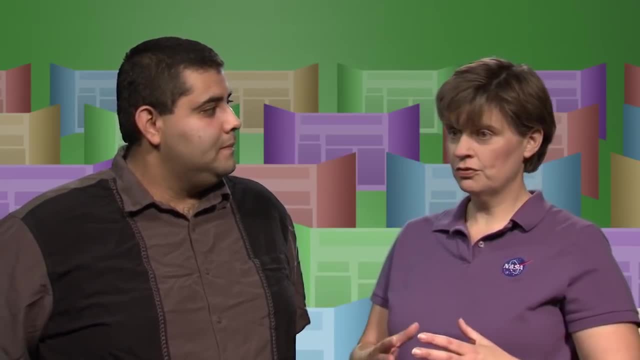 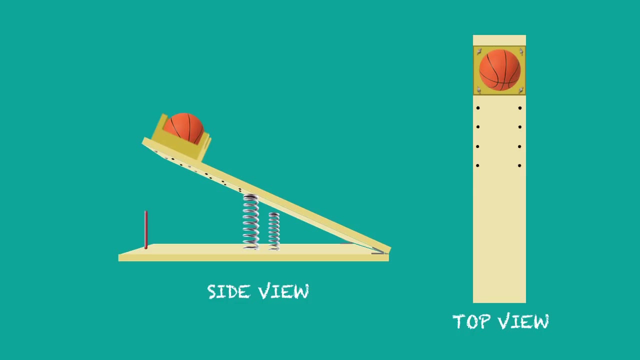 hardware store. you know what to buy Now. would you build a full-scale basketball shooter for the basketball hoop on the side of the building, or would you build a small one? That's the great thing about designs: that they're scalable. You can. 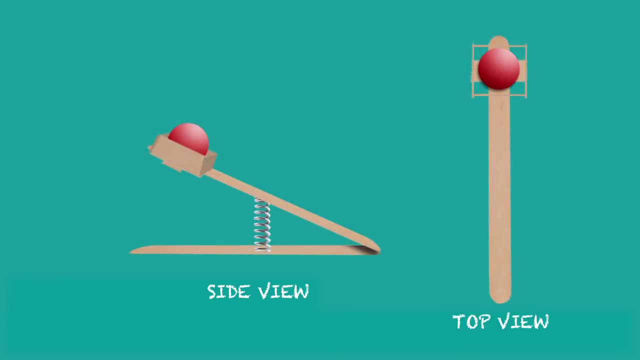 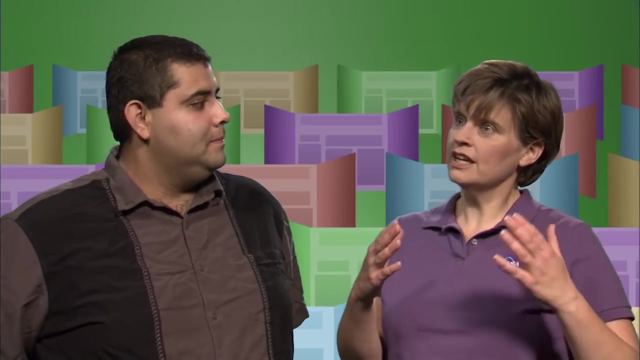 You can start out by building one out of Popsicle sticks at a small scale. make sure it works, make sure you like it, and then you can move on to bigger and better things. with wood and larger springs, You could enlarge your design by using different materials. Could you also improve your design? 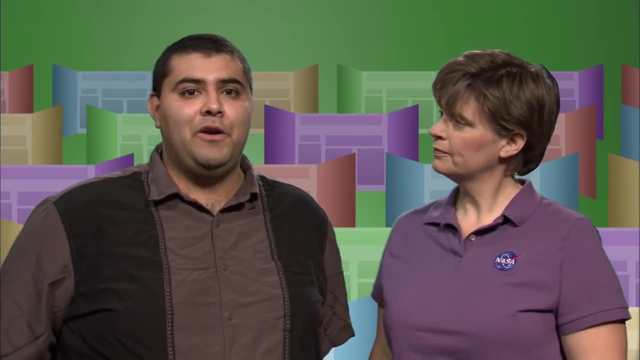 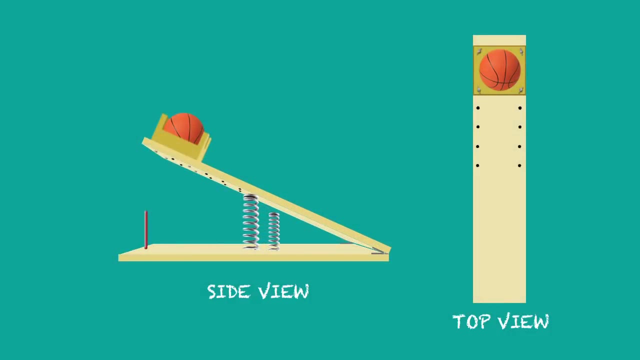 by using different materials. Yes, One of the big things in engineering is always wanting to make things bigger, better, faster. So once you move from Popsicles to wood, next thing you want to do is performance. Maybe you start out shooting at fifty percent with this free throw machine and you want 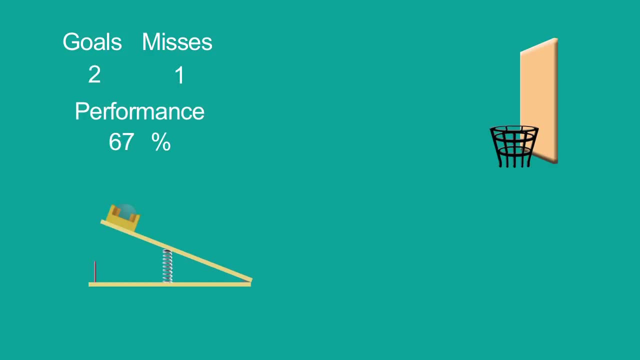 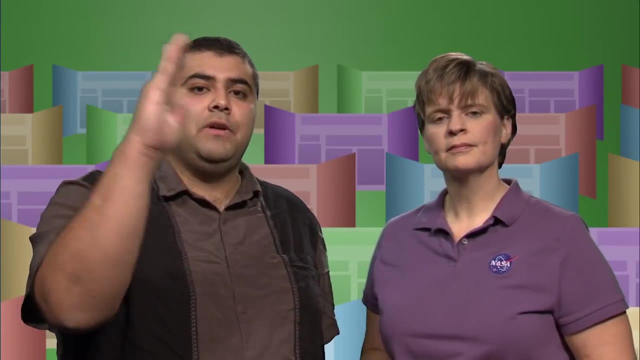 to get it up to ninety to a hundred percent. So there's a lot of different things you can do to improve the performance. One of the crucial things is the movement: How much force is the basketball going to be launched at and at what angle the ball is going to? 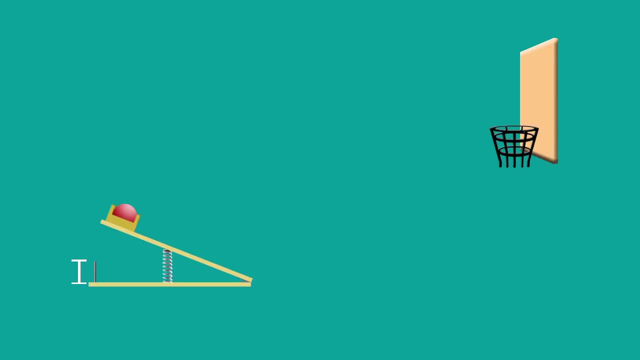 be released. There's a couple different ways to change that. The more you compress the spring, the more force you'll get out of it when it's released. So one of the things you can play around with is: at what level of compression do you get the basketball to? actually reach the hoop. There are different types of springs out there. Different springs. would that make a difference? Yes, Different springs, the amount of springs you use. The important thing in all of this is to run several tests. You want to keep the basketball holder at one position? then